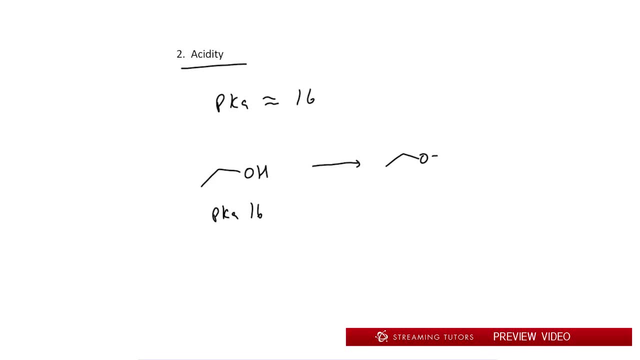 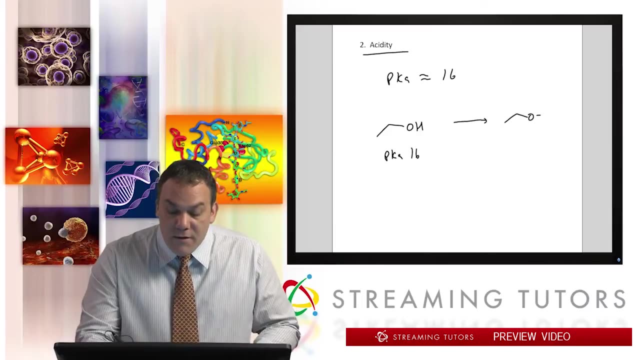 means that, whatever is on the other side, when this becomes an oxide and you have another acid, that that acid must be a larger number than 16, right, So this must be greater than 16.. And so there's only a few examples, So let's get started. So the first thing you should know is that a pKa of an alcohol is around 16, right? So in order for it to be considered an acid with pKa of 16, then that must be around 16, right? So let's get started. So, let's get started. So there's only a few examples. 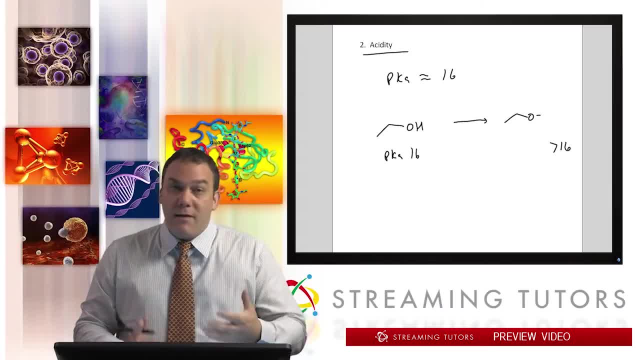 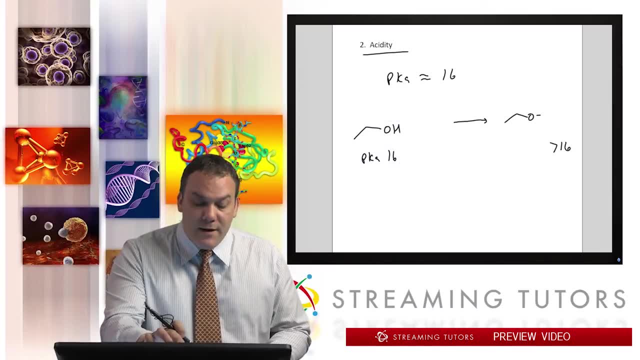 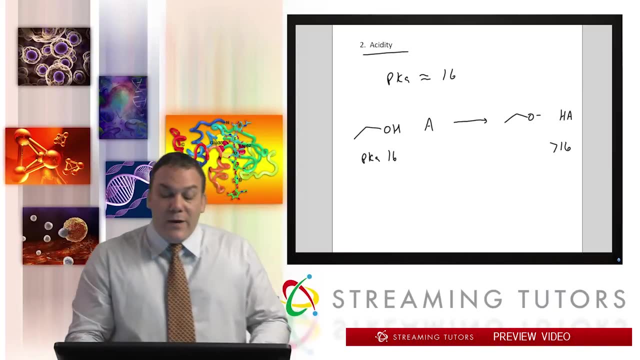 of this. It doesn't really react as an acid with many things. One most common example is if you have, let's say, a carbon, that's negative. So if I have A- I'll do it generically. then this becomes HA and we have to make sure it's greater than 16. So for A- it could be. 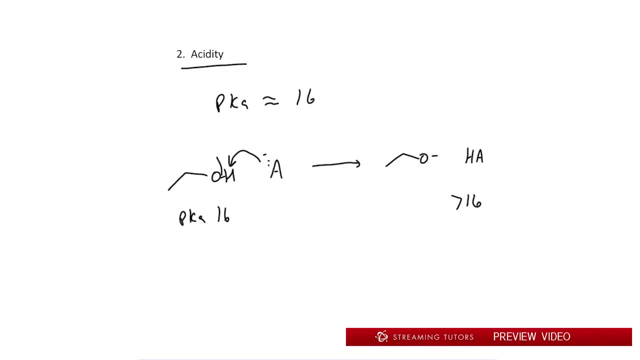 carbon. but what it does is it just pulls off the H and this becomes negative. So A- could be the following things: It could be a carbon like a R that's negative. Now, usually that's with a metal next to it, like methyl lithium is an example of that. Or you could. 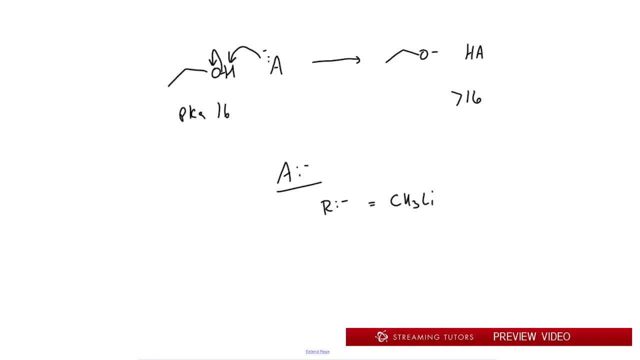 have alkenes or alkynes, right. So we can have an alkene that's negative or even an alkyne that's negative, And they all become acids that are higher or greater value than 16, okay, Now another one is. 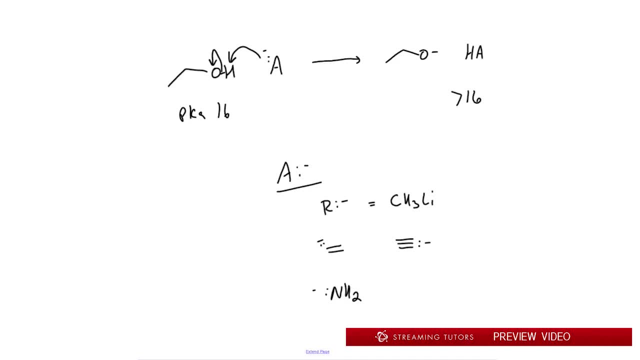 NH2.. This is a good base. It becomes NH3 when it gets protonated. So this right here is a base. I'm not going to write the NH3.. I don't want to throw you off. These are the bases that we can use. 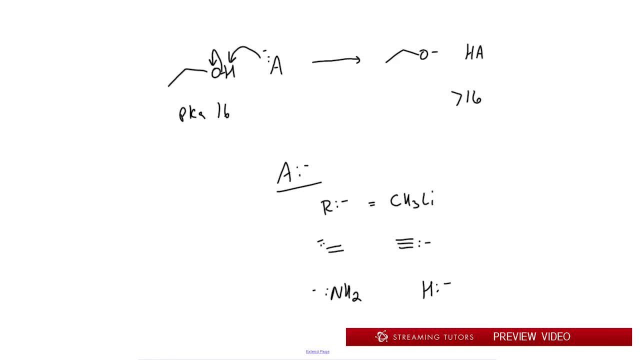 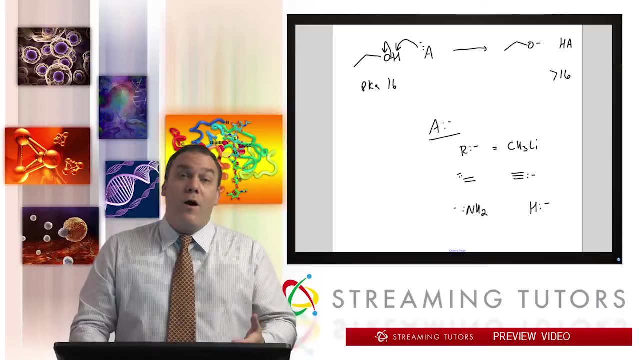 H- or NAH, same thing right. A lot of times, when things are negative, you have a metal to disguise its negativity. It counters it. So NAH or LIR or NAH2, these are things that will get protonated. 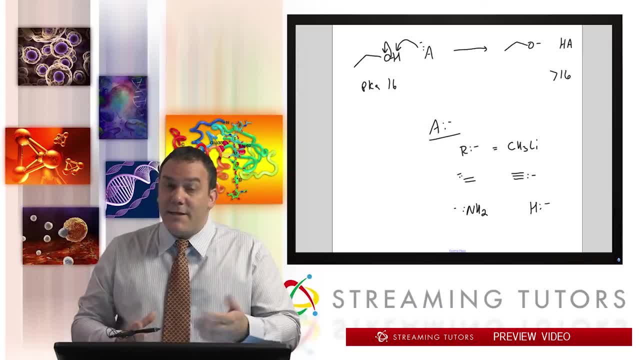 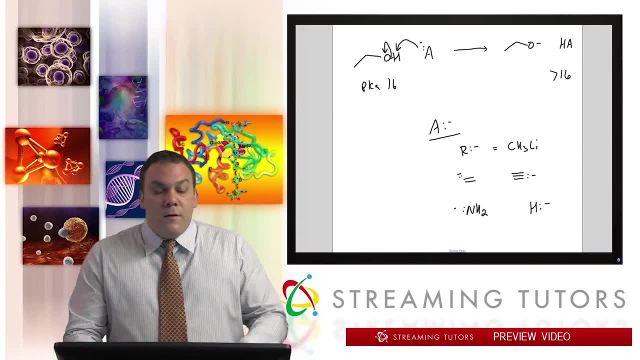 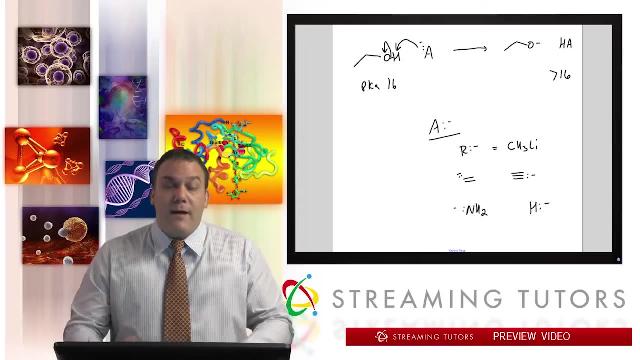 by an alcohol, Because they're all pKa value. the conjugate acid of these are higher values, higher pKas than alcohol itself. So these are the most common ones And this really comes down to the most important ones for you. So just keep in mind any carbon right Other than, for example, CN – that's not going to be an 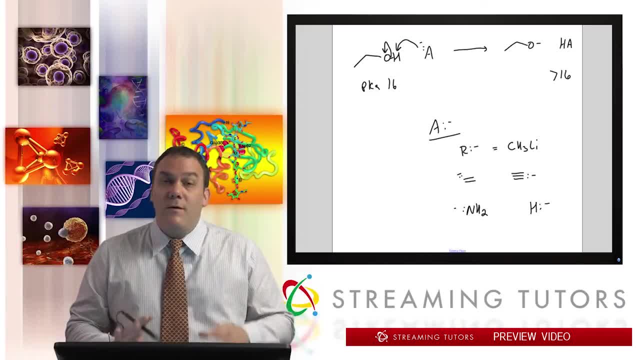 acid-base reaction with an alcohol. It won't be a base with an alcohol, okay. But carbons that are not positive, meaning they don't have like a nice stopped state, okay, They just retain tension Like that's already not a positive. So, Bürger, Alkene, like I've mentioned, c rinse motor rightants Want to one time. see. if this happens, It's go och okay. Well, you get the impossible together. So you always have to pick that thing right. Here are the all basal and you'll have to get pregunta to the answer. I'm saying you know. 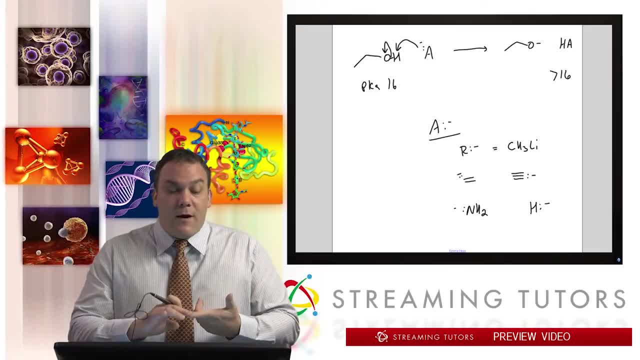 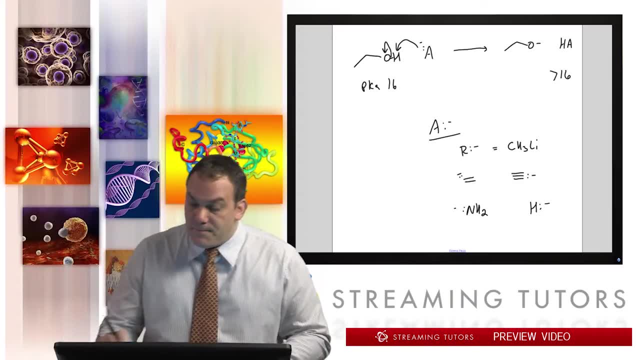 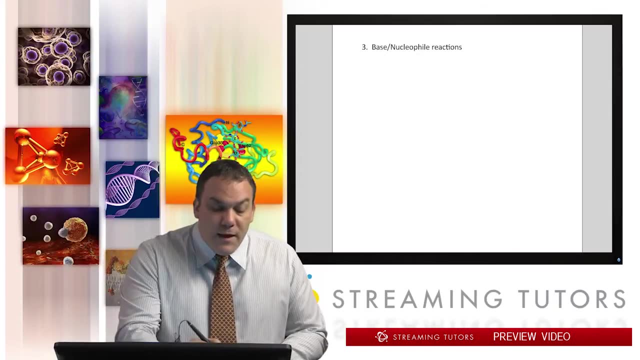 like electronegative groups next to it. So things like carbons, like sp3 carbons, sp2 carbon, sp, carbon hydrogen and nitrogen. Those are the ones you should keep in mind Now. also, alcohols can act as bases or nucleophiles. So when we talk about nucleophile, 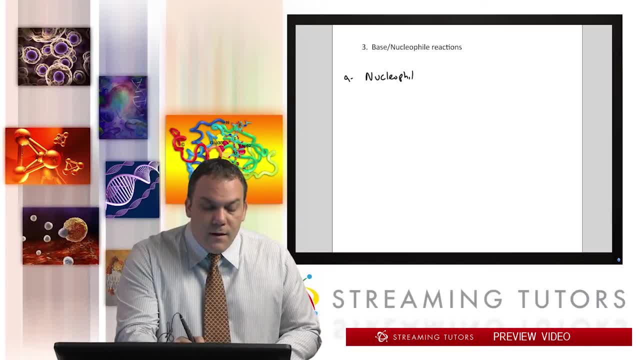 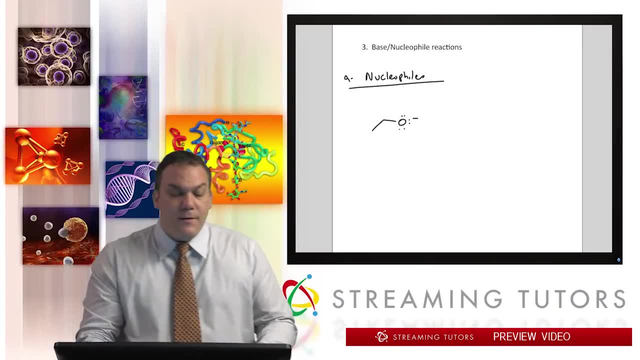 we'll write A for nucleophiles. Remember the nucleophile. what that simply means is that you have an oxygen. usually it's negative, but it doesn't have to be. If an oxygen is negative and it's not going to grab a proton, instead it's going to attach onto something that has a 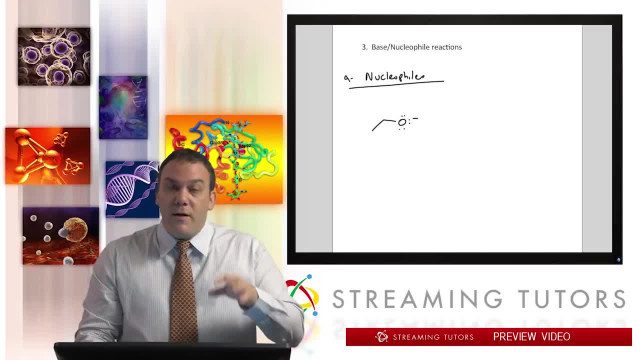 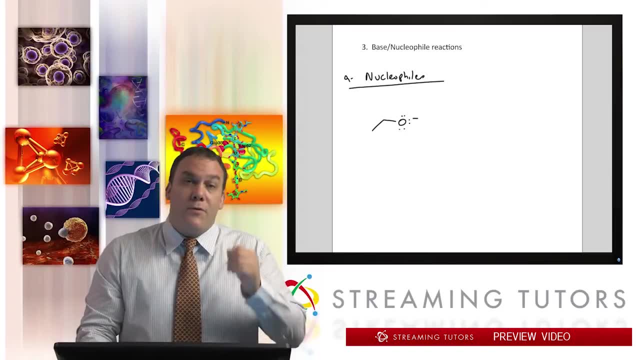 leaving group, then it's a nucleophile, right? So remember, nucleophile is a kinetic term- It's more about the rate, the speed, not so much stability- whereas base is a thermodynamic term- right, That's more about stability. In our case, we're going to talk about nucleophile. 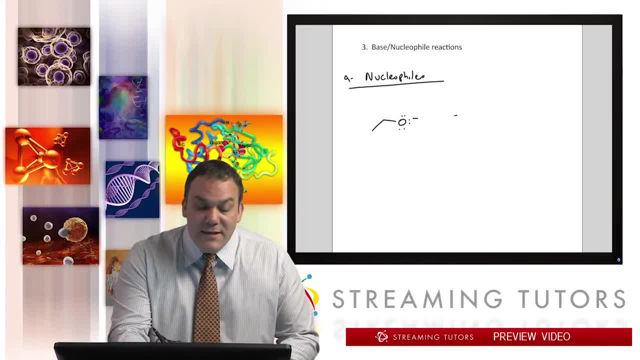 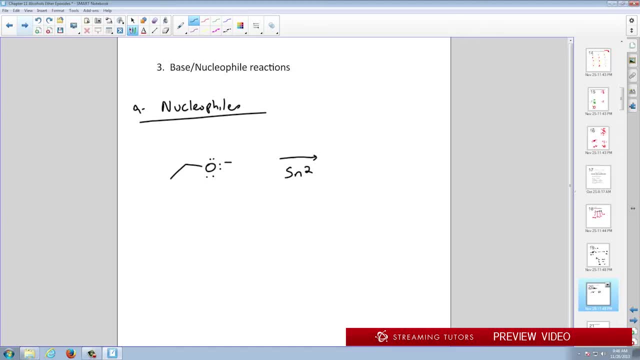 So if you have an oxygen as a nucleophile, if it's negative. if this is negative, then SN2 is favored for substitution. And so how do we do that? Well, the R group must be equal to either methyl or primary, and then the oxygen will act. 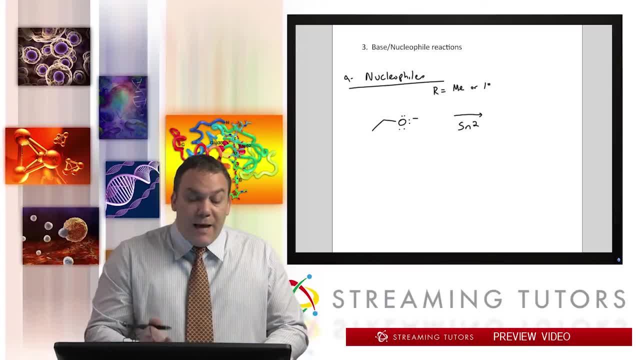 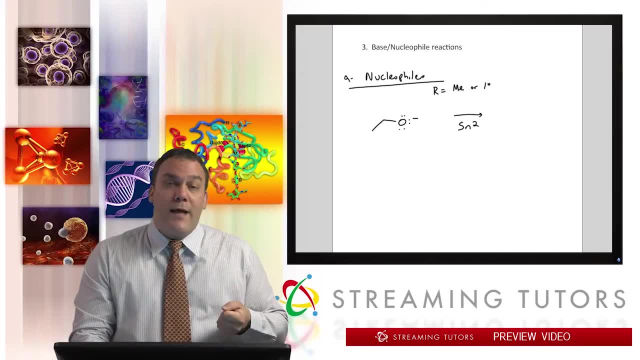 as a nucleophile. So what we can do is, for example, we can have a neutral alcohol and we use a base like NaH, for example, to pull off the H from the alcohol and then it acts as a nucleophile. 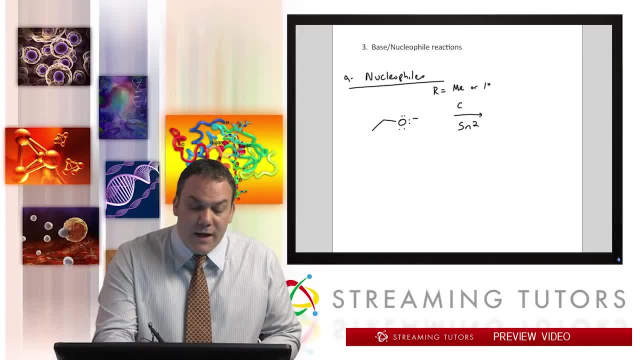 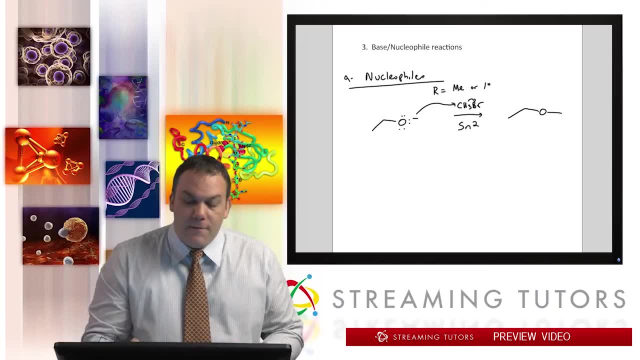 It goes after something. So in our case we can have it go after, let's say, methyl bromide. So then that would come in SN2, this leaves, and you're done. You get to this right here. Now, if it was higher than primary, then it's probably not going to go through SN2,. 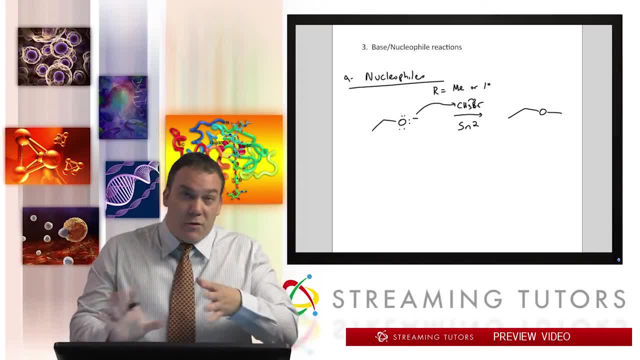 it's going to go through E2, right. So that's why we kind of keep it at methyl primary for the alcoholide side. Now, of course, the halogen could be BR, CL, IF any of the halogens that we've 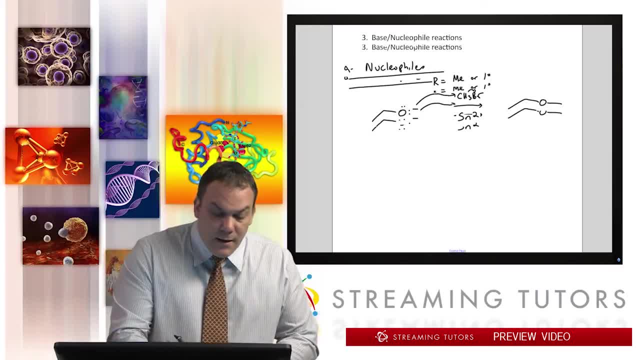 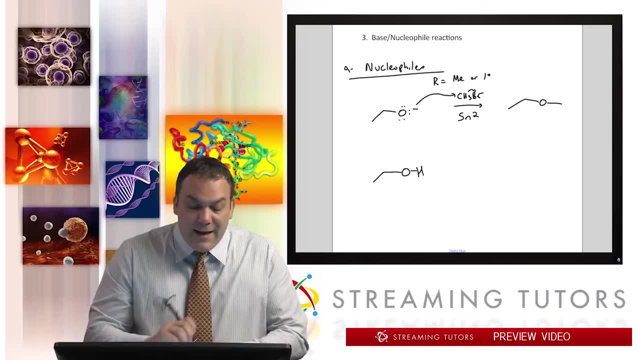 talked about all semester long. Now, another possibility is where we have an alcohol and we don't make it negative, We leave it neutral, and in that case we want to go through an SN1 reaction. So when it's neutral, 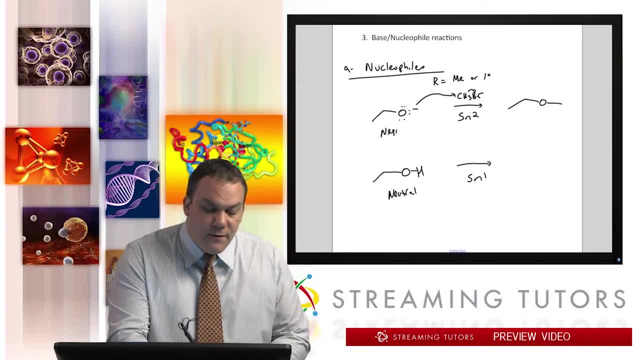 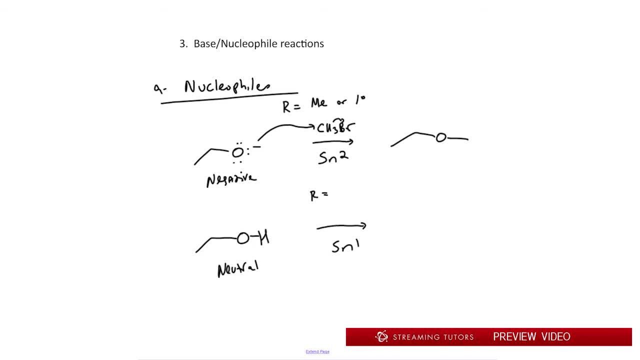 then it's favoring SN1.. If it's negative, it favors SN2, not SN1.. Now with SN1, the R group should equal tertiary or secondary. Now if we have for example, a tertiary alcohol bromide, then this is going to go and attach on to the tertiary carbon. 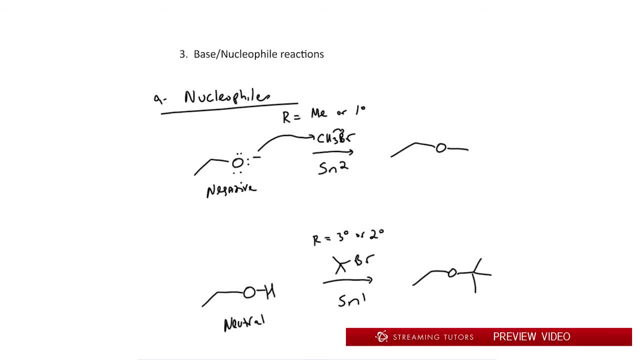 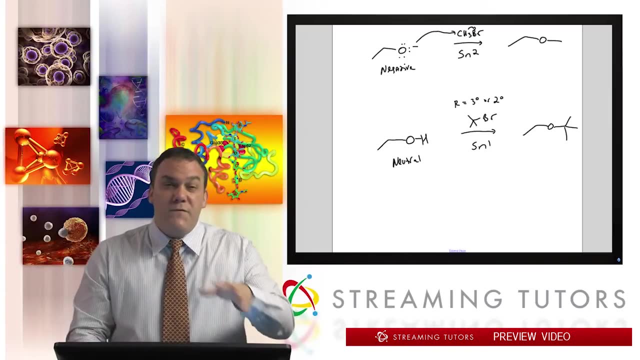 like that, And that would be SN2, sorry, SN1.. So what's happening here? the BR is leaving, carbocations forming and then oxygen is coming in. I'm not going to go through the full, detailed mechanism, this mechanism, many times, So I just want to give you the general overview. Now another one. 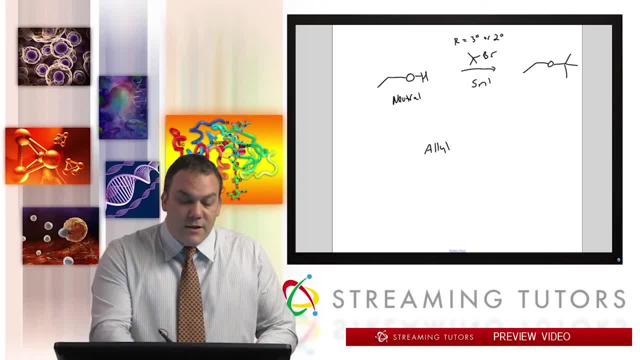 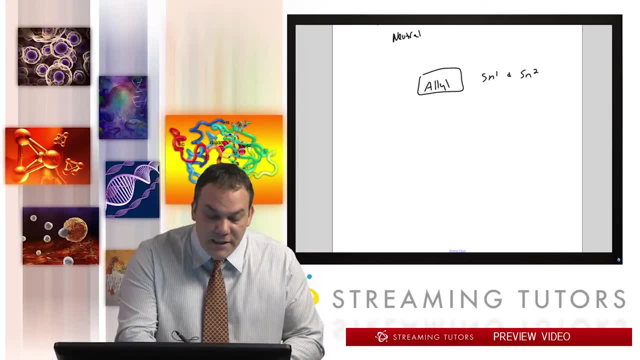 that actually favors both allyl is going to favor both SN1 and SN2.. Okay, so it depends on the degree of the allyl. So, for example, if I have an alcohol and I treat it with, let's say, an allyl, 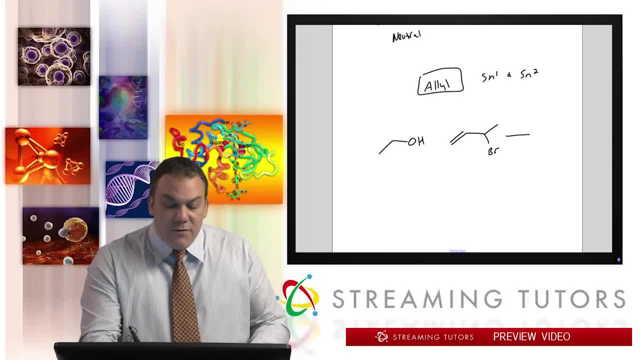 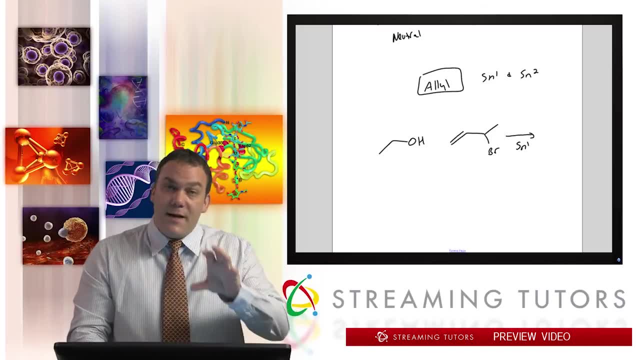 and then it has like a BR right there. well then, this right here is going to go through SN1.. The reason why I say that is because the alcohol is neutral, right, It's not negative. So that tells me SN1 is favored over SN2.. And the fact that this is actually- let me make it primary- 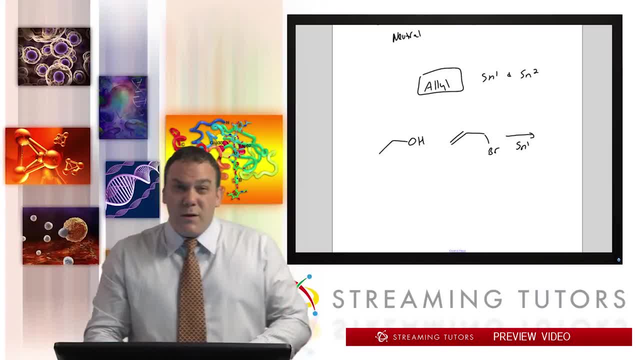 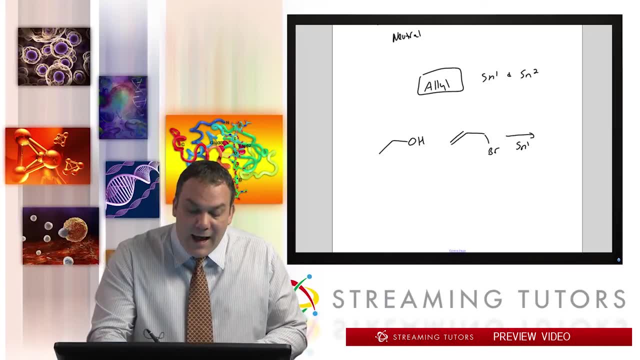 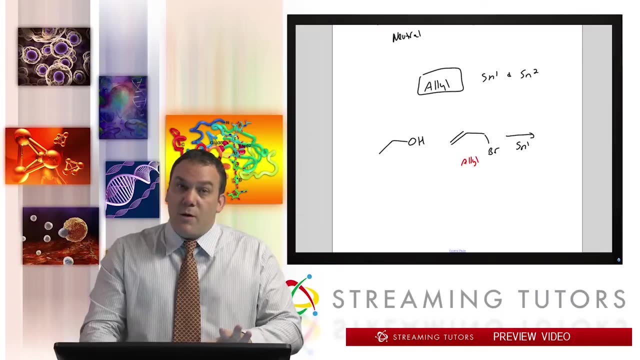 so I can make my point. So this is a primary, which normally you would think is SN2 for primary right, But the fact that it's not really just primary, this is allyl right. This is a carbon that's next to a double bond, So this will go through SN1.. So this is unusual. So I want you. 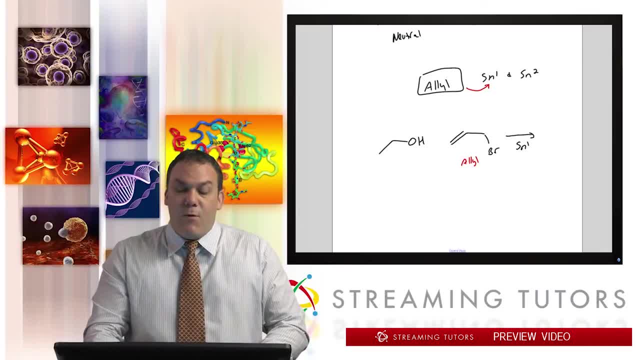 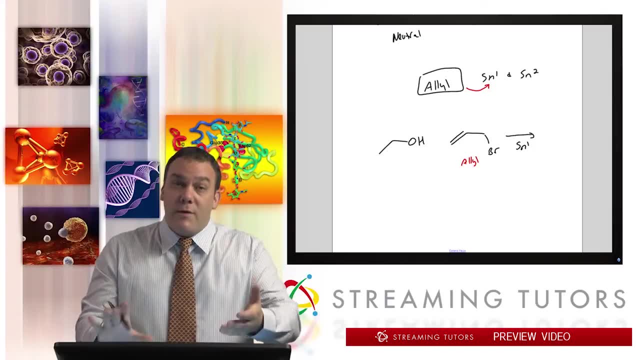 to think of allyl as something that can definitely go through SN1. It could go through SN2 also, but if it's neutral, it's going to go through SN1. If it's negative- the oxygen- it would go through SN2.. But here's how it works: The BR leaves and you make a carbocation. 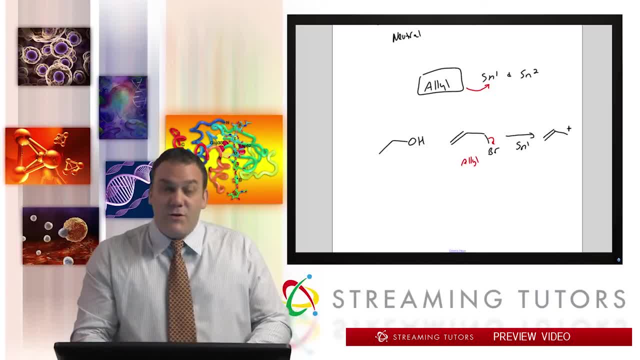 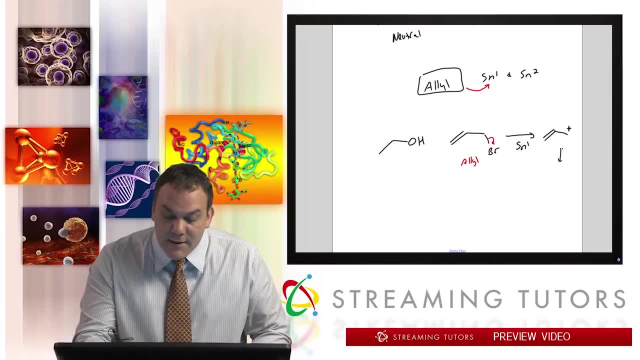 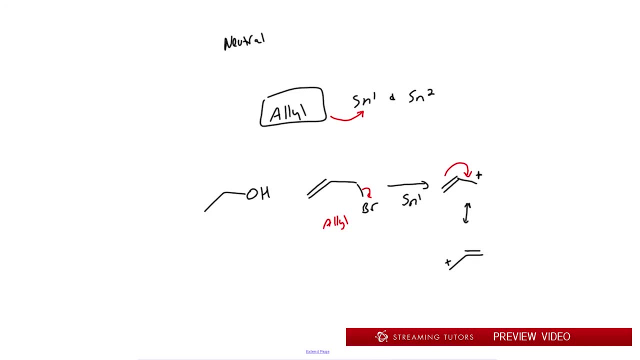 And because that carbon that's positive is really not just primary but it's next to a double bond. it has resonance stabilization right. So this has resonance stabilization, which means that the The double bond would go here and the positive's on the left. So because allyl has this characteristic, 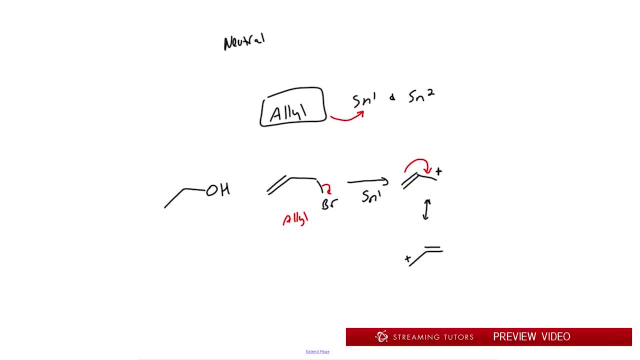 to it. it is very reactive. It's very good to do this. It's faster than tertiary okay, So not always, but in this case it would be. So allyl is a very good position for a carbocation, And so 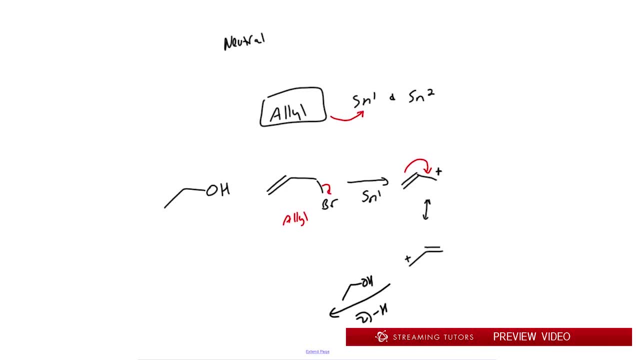 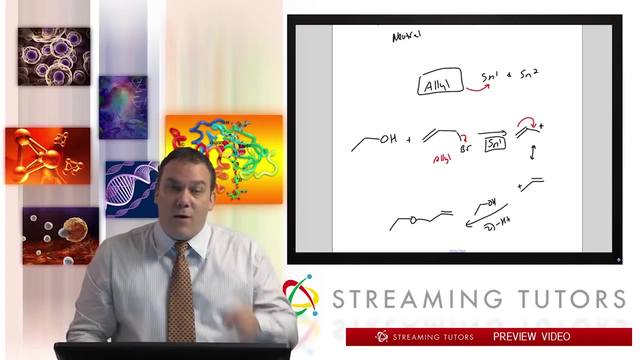 therefore, when the alcohol comes in, step two is minus H+. we will get oxygen to attach on like that. okay, SN1 favored reaction. Now again, if the alcohol that we were using was negative- if it was an oxide RO- then SN2 would be favored okay. So keep that in mind. So nucleophilic attacks occur when it's methyl primary SN2, even if it was alcohol neutral SN2, because it's low degree, you don't want to make a carbocation that low If it's high tertiary secondary and it's neutral oxygen SN1.. Now you might say well: 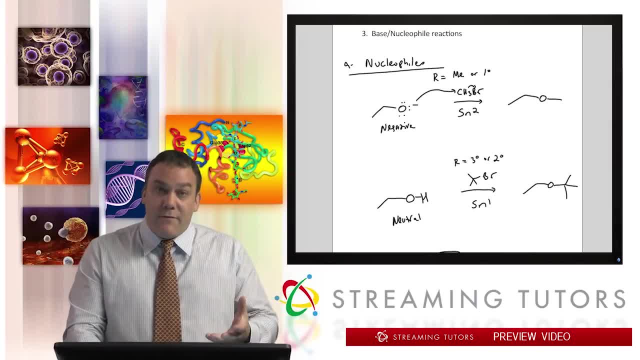 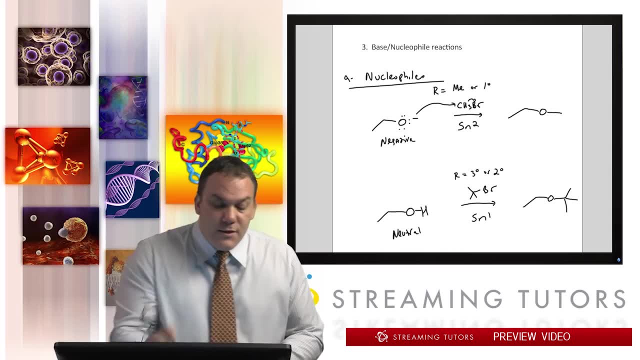 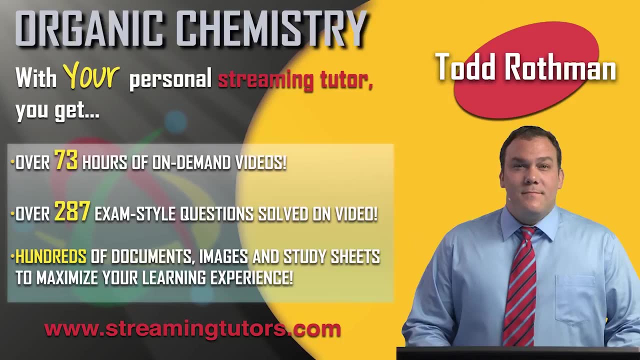 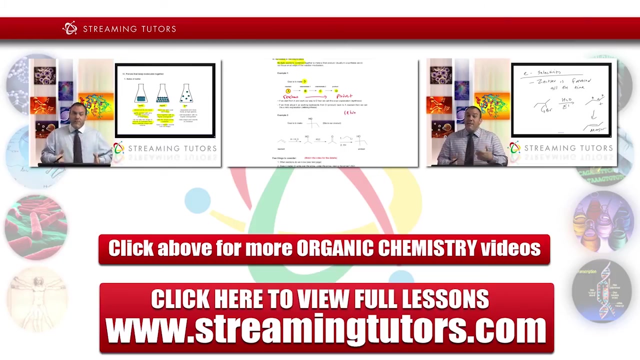 what happens if it's tertiary or secondary and it's negative oxygen? Well then, that goes to E1, okay, That's elimination. Let me review that with you. So this is nucleophile. Now let's talk B. This is the E1.. This is D1.. So at this point we're going to go to average. So, Boss. 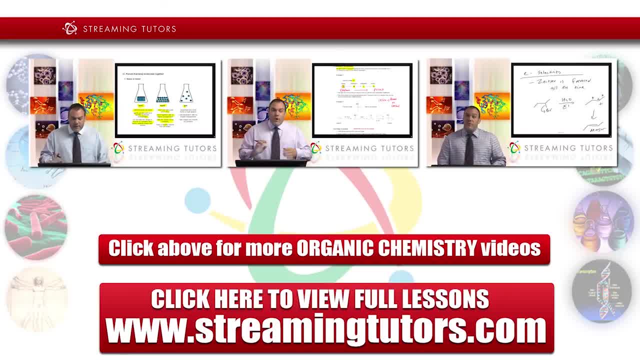 I spoke about it. B is A. It's a relatively low B A. it's C, it's D, But allyl is normal. It's normal in the case of the B is C. So that was my conclusion, because this is the. this is. 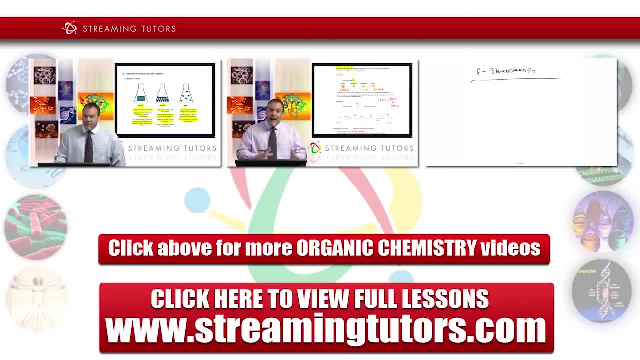 the case of the life of a student, And I would say it's not the case, because you know we are getting into, you know the shit we're from here, you, you.